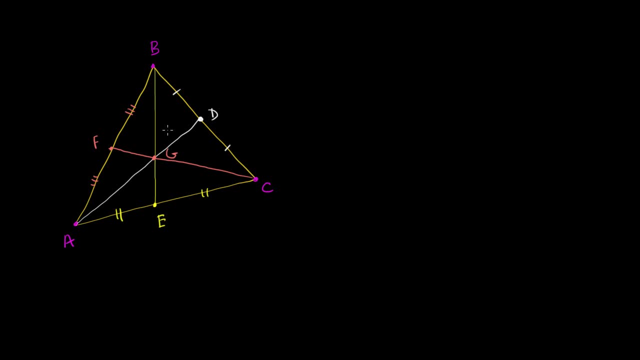 And that's what we're going to prove in this video- that these six triangles all have the same area. Now, to start off, I'm just going to look at different pairs of triangles, So let's look at these two triangles right over here. 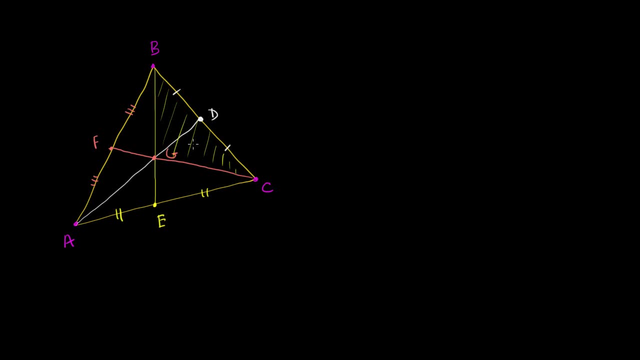 Let's look at those two triangles over here And to show that those two have the same area, we're just going to invoke a very simple principle. So imagine rotating just those two triangles over. It would look something like this. Let me try my best to draw it. 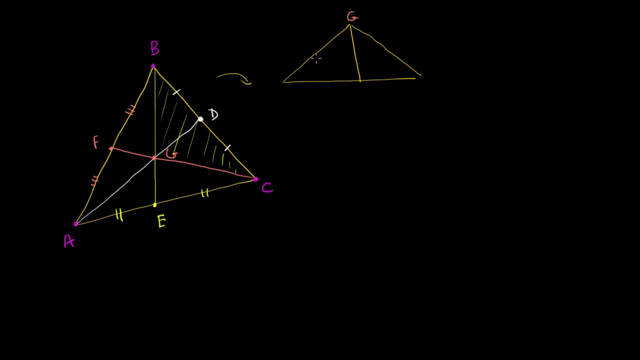 Where this would be point G. I'll even try to color code it the same. That is point G. That is that side right over there. This is point C. This is point B. That is point B. And then this right over here would: 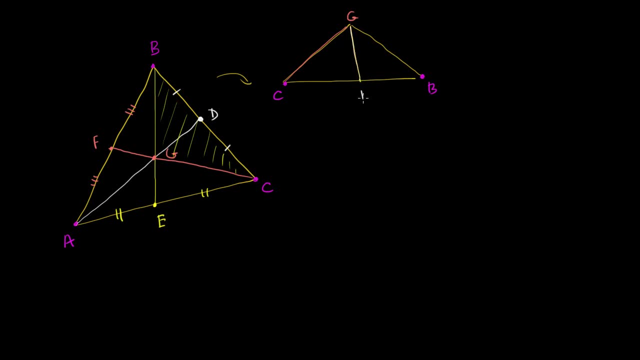 be the second part of that median right over there, That over there would be point D. Now we know- and I didn't draw it actually that nicely over here- we know that this length is equal to this length right over here, That these two triangles, if we're 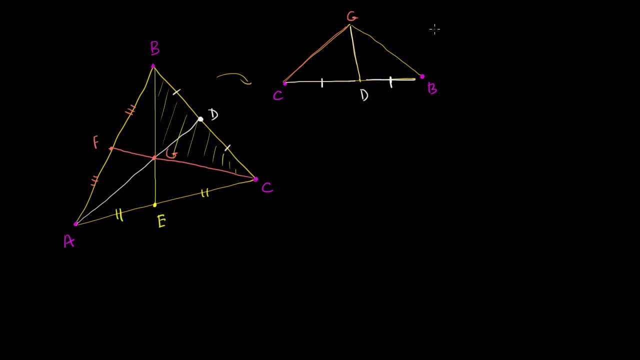 starting to think about the area. they have the same base And we know area is equal to 1 half base times height. So they definitely have the same base. What about their heights? Well, they also have the same heights. Both of their heights is exactly that tall. 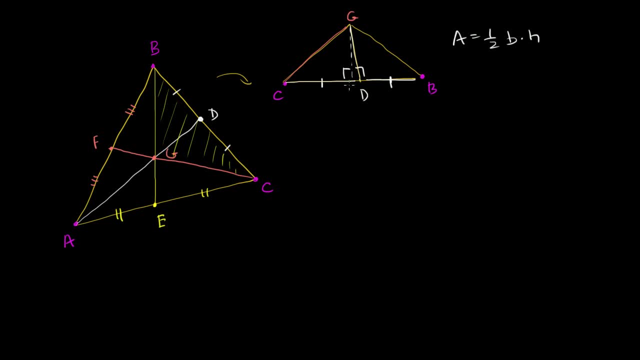 They both have the same height, So both of them have the same base. They both have the same height. On an obtuse triangle right here, the altitude sits outside of it, So that might be a little counterintuitive. So if you have an obtuse triangle like that, 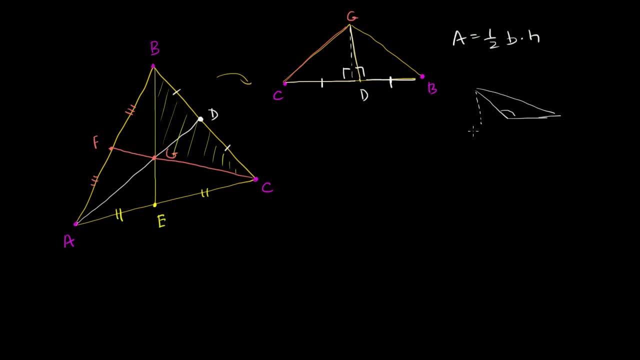 I say obtuse because this is more than 90 degrees. your altitude, your height will actually sit outside of the triangle, But that's OK. Both of these triangles have the same base and the same height, So they must have the same area. 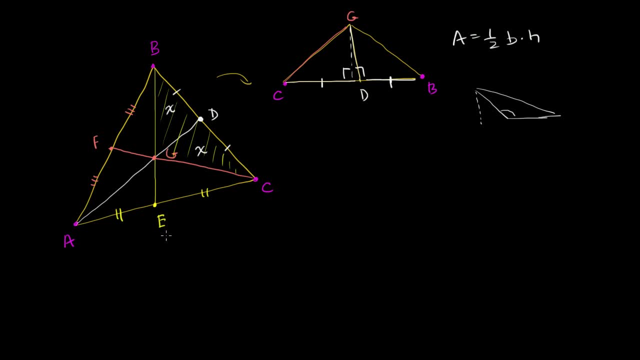 So if this one right here has area x, this one right here will have area x as well. And you can use the exact same logic to say: well, look, This guy and this guy, they have the same base And they both have the same height. 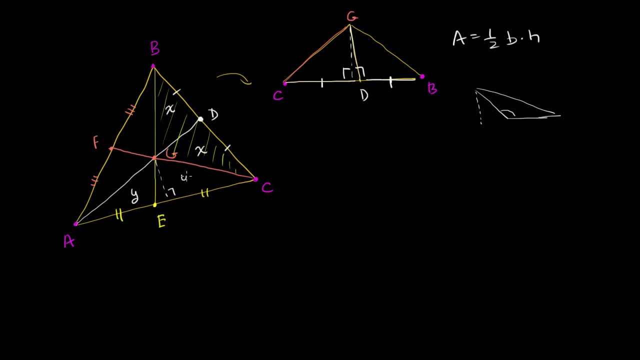 So if this one right over here is the same height, this one right over here is of area y, then this one over here is also going to be of area y. They're going to have the same area, And then, finally, we could do the same thing. 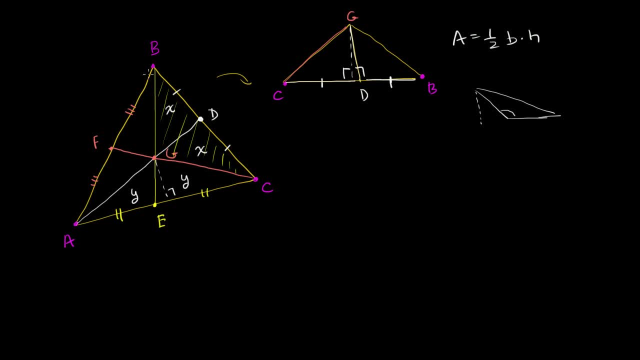 for these two characters up here. They both have the same base. This was bf, is equal to fa And they both have the same height. We drop an altitude like that, And so if we call this area right over here z, you could call that area z as well. 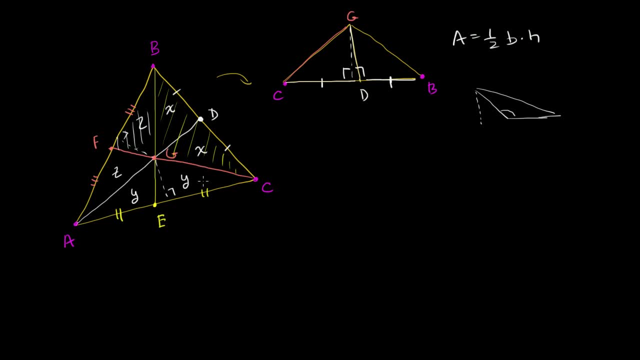 So so far we've shown that we can divide this into three pairs of triangles that have the same area, But we want to now show that they all have the same area, And to do that we can invoke this same principle, But we'll do it with different sets of triangles. 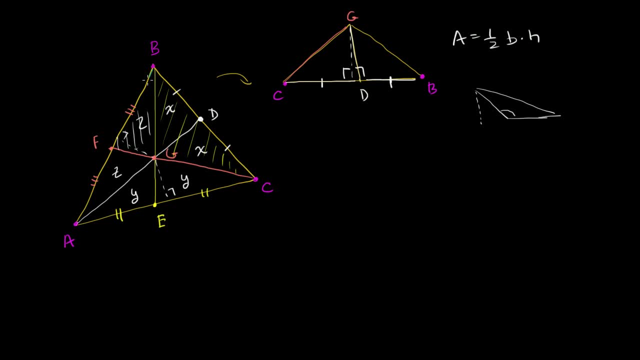 So now let's look at triangle bae. So the area of triangle bae is going to be equal to z plus z plus y. And let's look at the area of triangle bec right over there. That's going to be this triangle right over here. 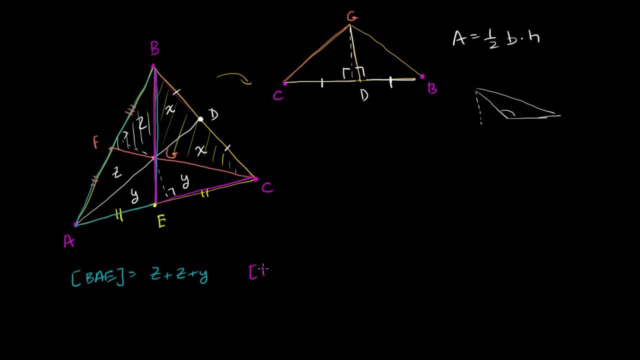 is going to be x plus x plus y, So the area of bec is going to be x plus x plus y, But this same principle, they both have the same base And they both have the same height. We could drop an altitude like this. 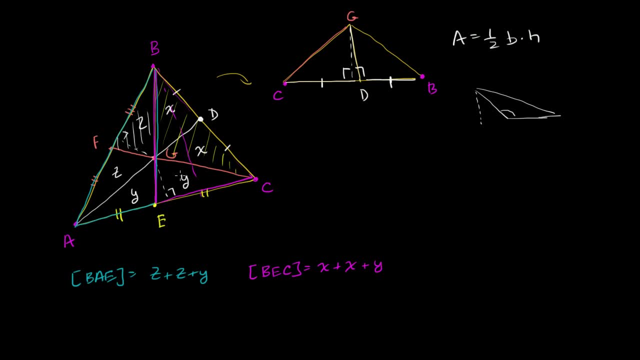 This one is obtuse so that the altitude sits outside of it, But they have the exact same height. These two areas need to be equal to each other. So you have z. well, let me just add that up that you have. 2z plus y is going to be equal to 2x plus y. 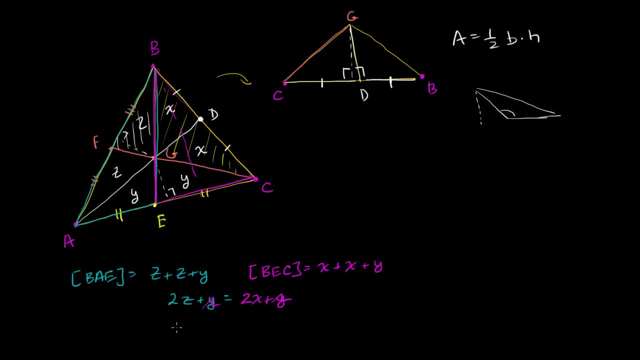 Subtract y from both sides, you get 2z is equal to 2x. Divide both sides by 2, you get z is equal to x, And so we could write an x here and an x there. So we know that all of these four have the same area. 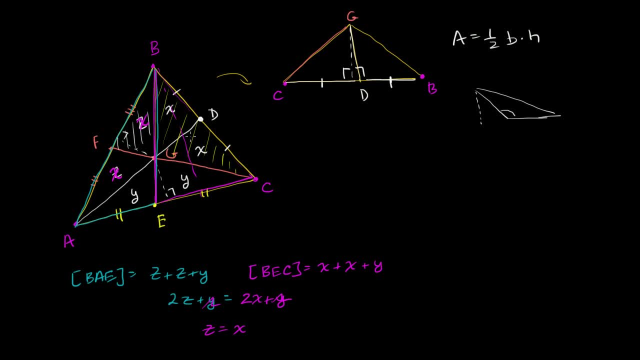 But we still have to worry about these y's here, And to do that we just have to kind of rotate the way that we look at it. And now look at triangle adc. Let me do that in a different color, Triangle adc, which I'm highlighting right over here.